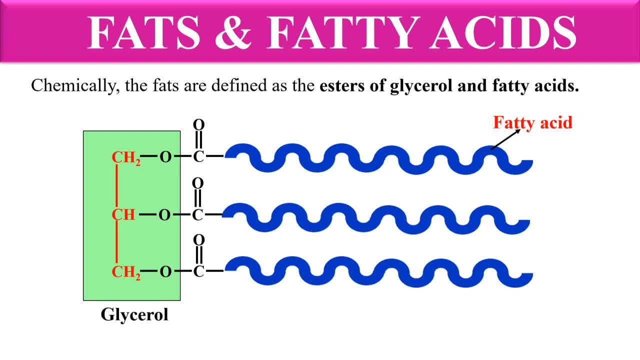 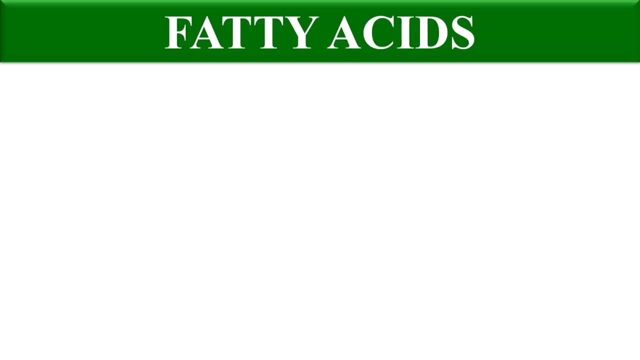 So you can simply say the fats. The fats are the triesters of glycerol and fatty acids. Now let's discuss about these fatty acids. So fatty acids, these are the organic acids which have carboxyl group at one end and they have a long- you can say- hydrocarbon tail. 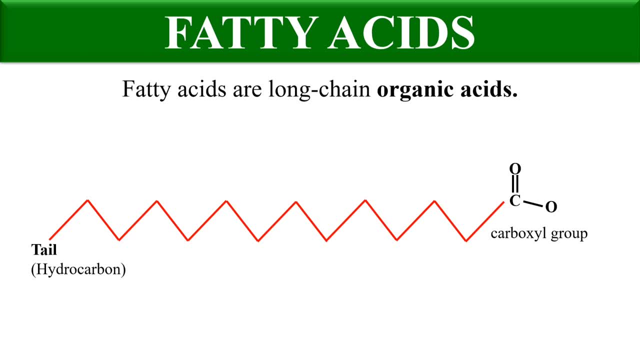 Due to this tail, they give hydrophobicity and oily nature to the lipids. So this is the structure of typical fatty acid, in which you can clearly see carboxyl group at one end and which, from this, there is a run of long hydrocarbon tail. 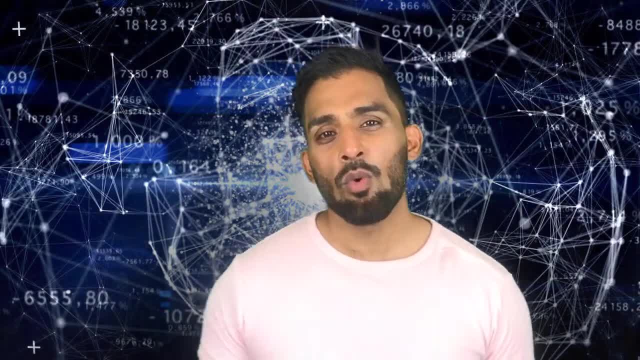 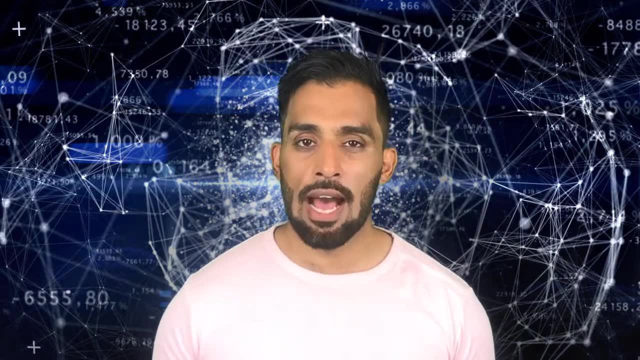 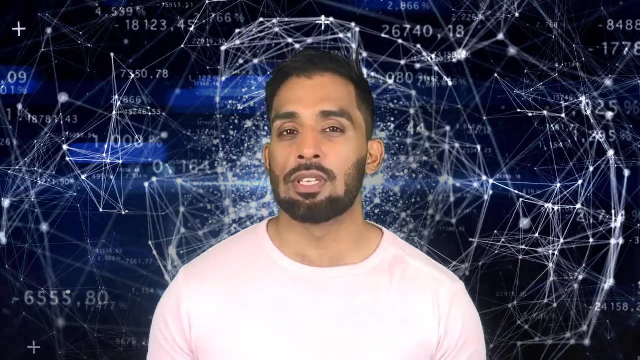 Hey, welcome to another episode of 5-Minute Computer Science. My name is Mr K and today we're going to be looking at memory management. So how does the CPU manage memory and how does the operating system work with the CPU in order to keep your programs running, your 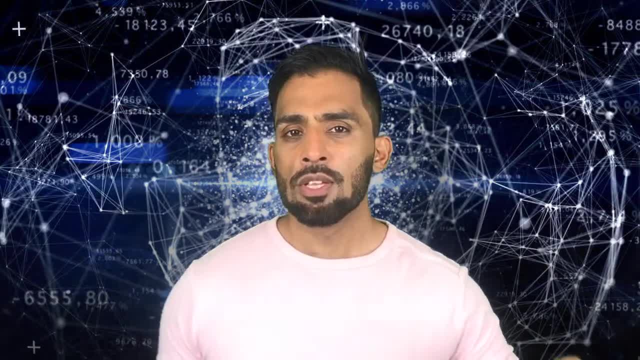 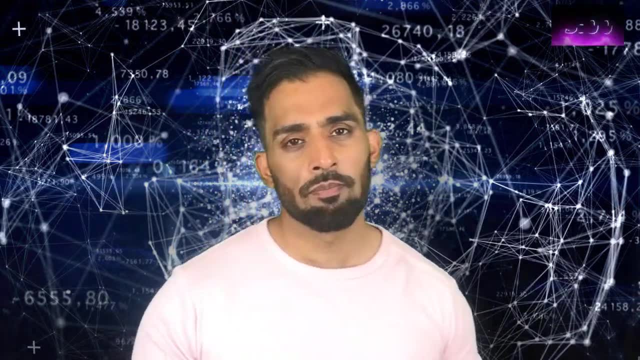 downloads, downloading and everything to run smoothly. So we're going to be looking at things like paging and virtual memory segmentation and those kind of things. So let's put 5-Minute on the clock. Let's go for it, man. So let's have a look at an operating system and what 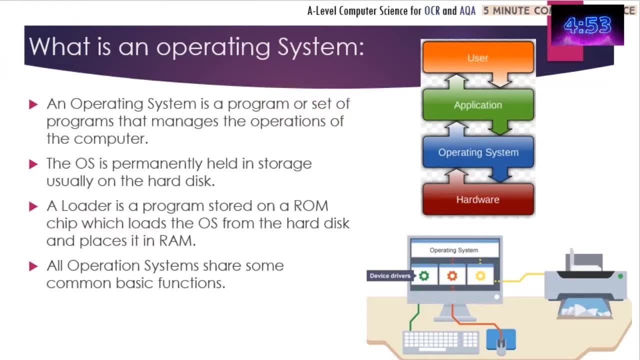 it does. Well, an operating system essentially is the go between a user and some hardware or a user and an application, And this can simply be understood like this: Assume you've got some work on a USB. Okay, you've got a USB, you've got some work on it, Well, you're. 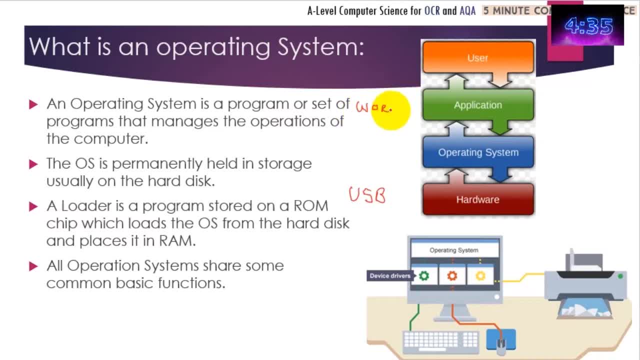 using an application. Let's say this is Microsoft Word, Okay. Well, how does Microsoft Word get a hold of it? Well, you've got a USB, you've got some work on it. Well, you're using an application. Well, it has to go through the operating system. So, the operating system.